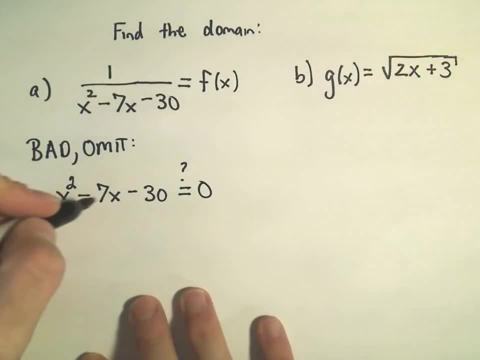 I'm thinking: what makes that equal 0?? Well, we just hopefully factor this. So let's see, I need two, I need an x and an x. to get my x squared, I need two numbers that multiply to negative 30.. 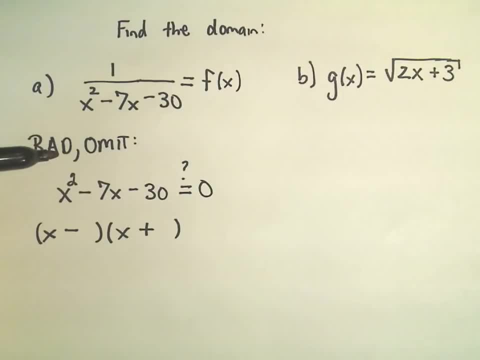 So I know I'm going to need a negative and a positive, Those two numbers. when I multiply them I have to get negative 30, but I have to add up to negative 7.. So I think if we use negative 10 and positive 3,, 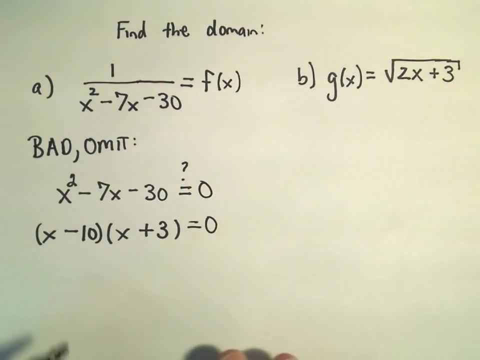 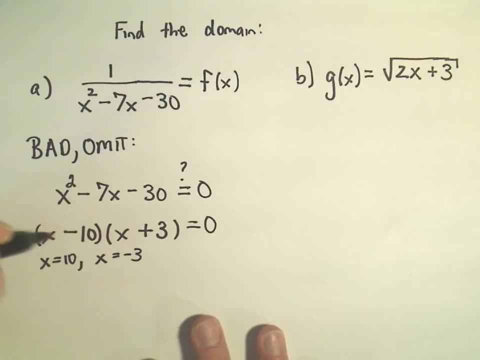 those two numbers will fit the bill And again, I want this to equal 0.. So if we set x minus 10 equals 0, we'll get x equals 10, and we'll get x equals negative 3 as solutions. 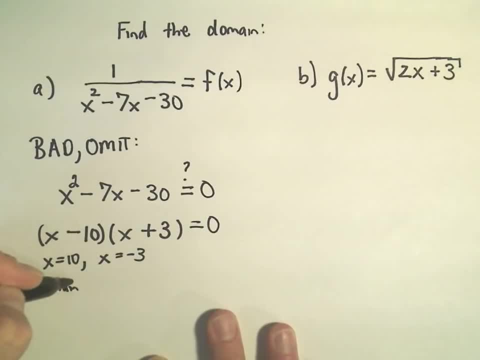 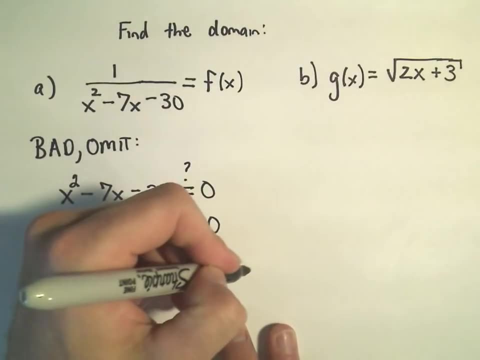 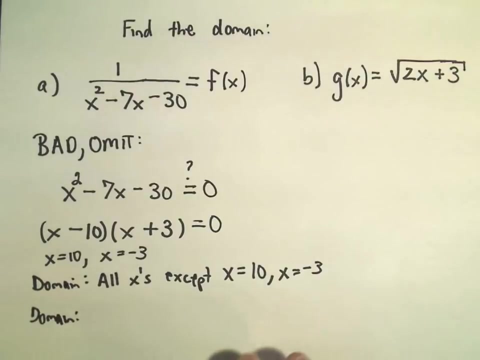 So our domain is going to be all values of x, all values of x, except for x equals 10, and x equals negative 3.. We could write that in interval notation by simply saying it's from negative infinity up to negative 3.. 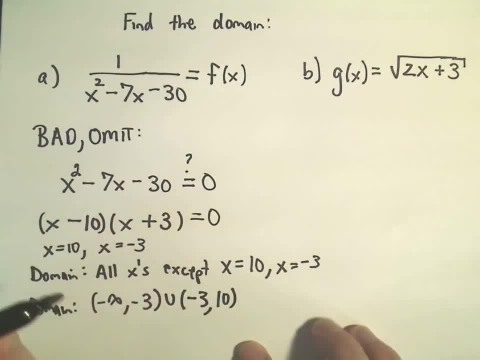 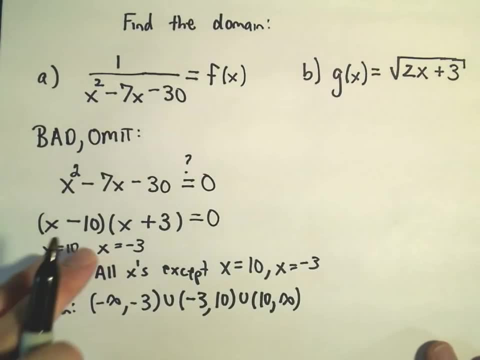 Then we have to skip over negative 3 and go up to 10.. And then we have to skip over 10 and go all the way to positive infinity. So sort of two different, equivalent ways. The other one: here we have the square root of 2x plus 3.. 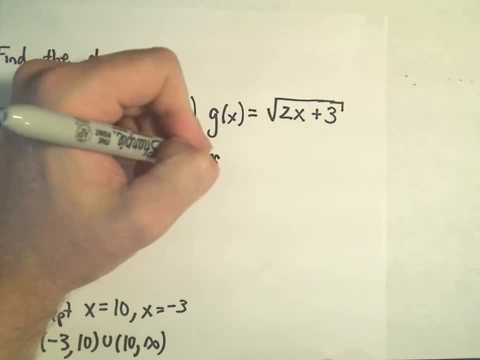 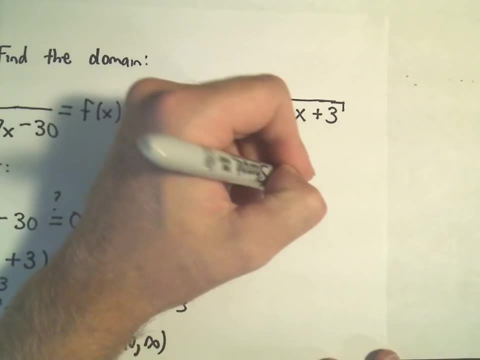 So again, to me, the values that are good in this case is the way I think about it. it's good if what's ever underneath the square root is greater than or equal to 0.. That's what we need to happen. 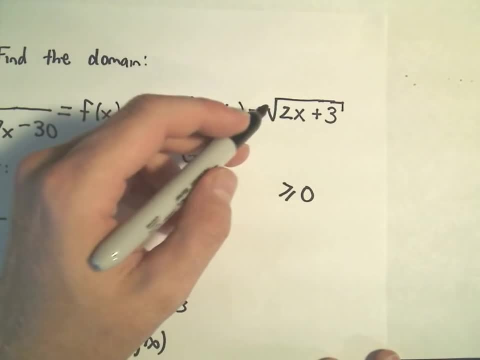 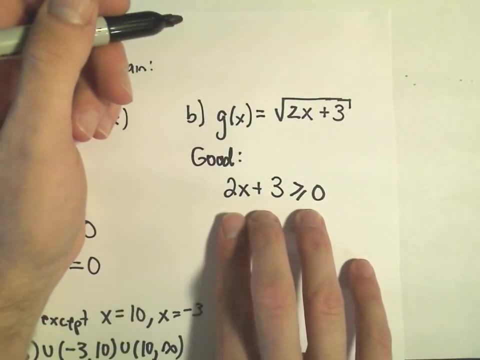 We only want numbers that are greater than or equal to 0, whatever's under the square root. Well, 2x plus 3, that's what's underneath the square root. So this now produces an inequality I have to solve. Unfortunately, this is just a linear inequality. 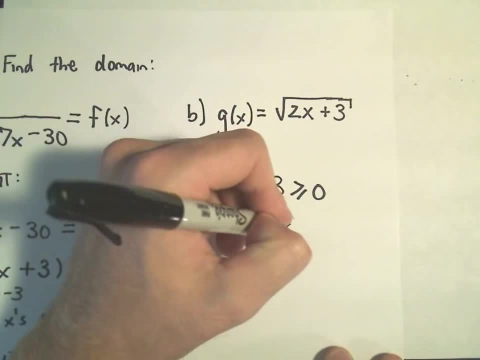 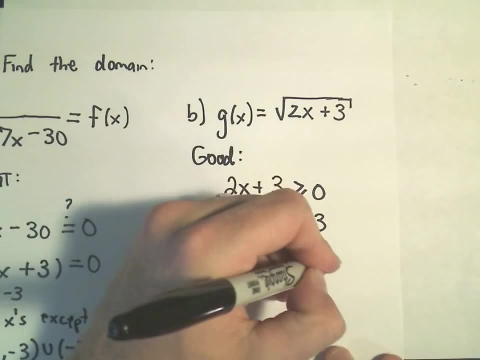 so it's not too bad. I can subtract 3 from both sides and get 2x greater than or equal to negative 3, divide by 2, and it says x needs to be greater than or equal to negative 3 halves. 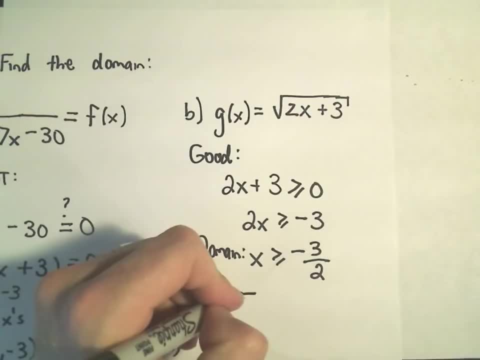 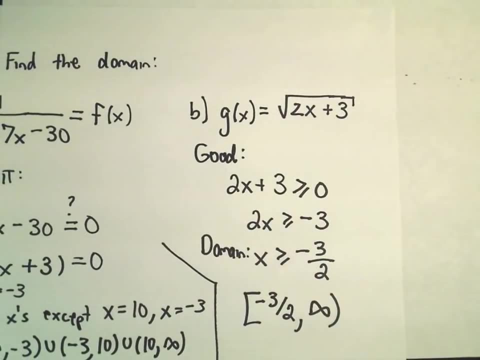 So again, this is my domain. in this case, In an interval notation we can write that, as brackets, negative 3 halves up to infinity, And that would be the domain for our radical or our square root function.